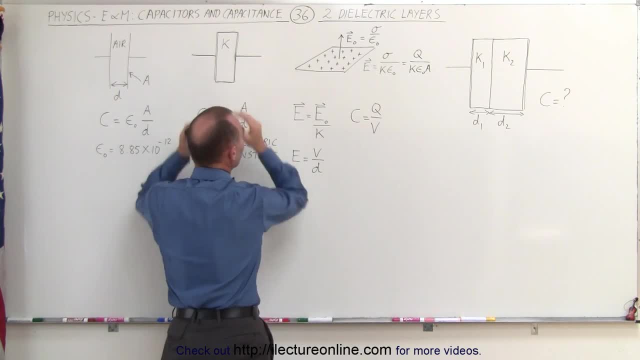 by the charge on the plates divided by the voltage difference between the two plates, and we also now, of course, can calculate the electric field magnitude as being the ratio of the potential difference between the plates divided by the distance. one more thing: we need to know that the electric field away from a charged plate can be calculated to be the charge density per unit. 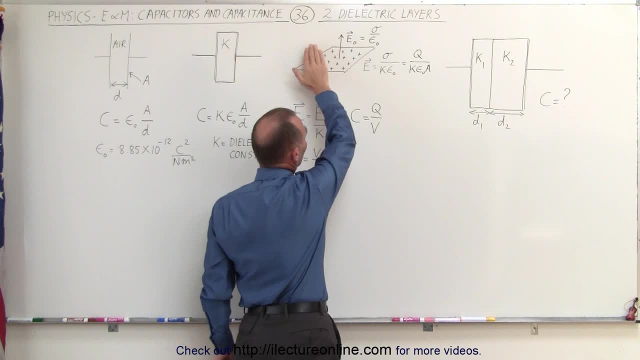 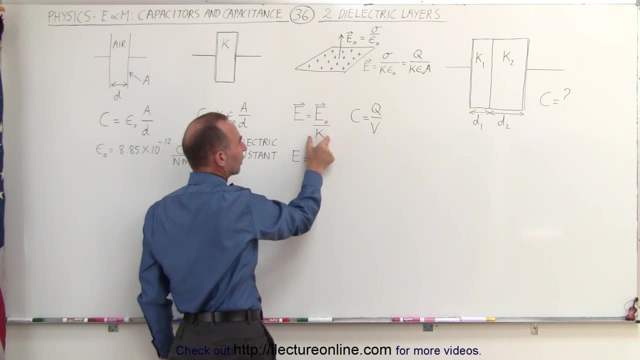 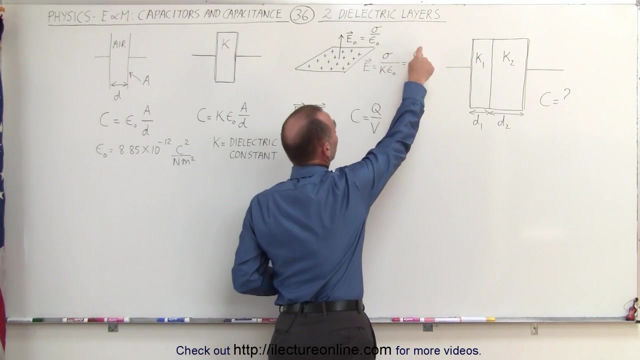 area divided by epsilon sub naught. or if there's dielectric on top of that, then we have to divide that by one over k again. you can see that the electric field is being diminished by the dielectric constant. so it needs to be done the same over there. and if we define the charge density by total charge per unit area, we can also 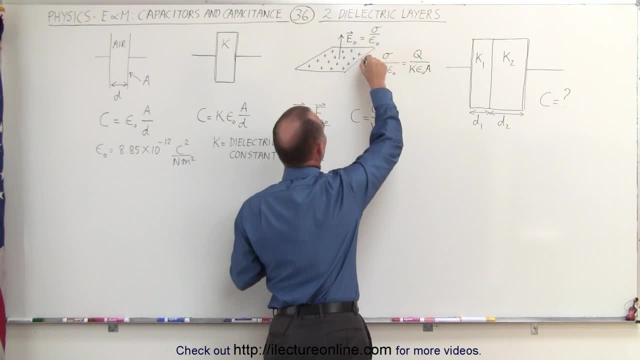 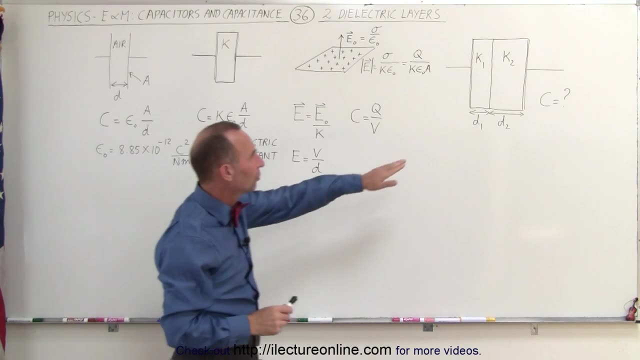 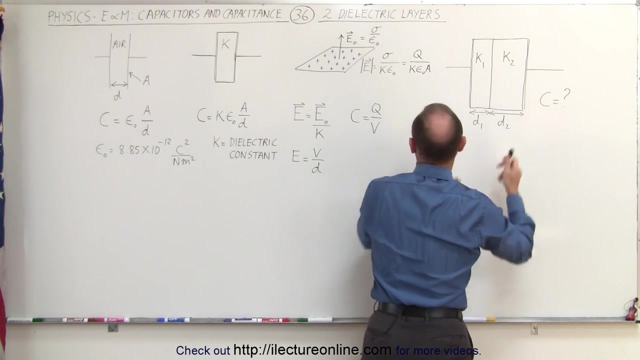 write the electric field like this, and of course i should put absolute value signs around it, because we're just giving you the magnitude of that. now, how do you find the capacitance of this? well, it turns out, if we can find the total potential difference here, we can then figure out. 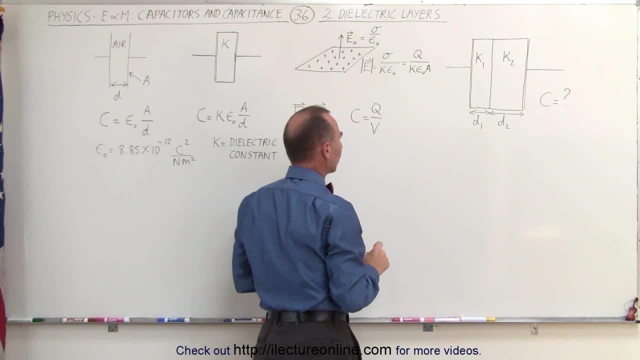 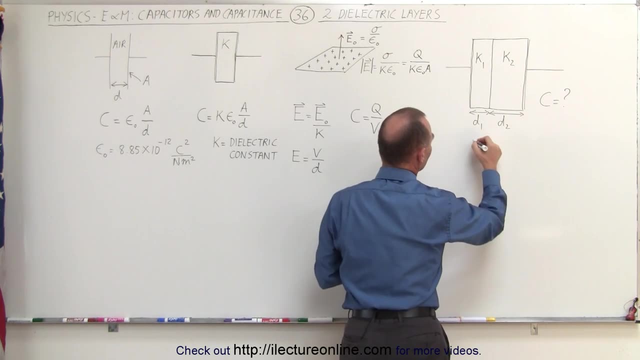 the capacitance by simply taking the charge divided by the potential difference. so what we can do then is realize that the potential difference will be divided between these two dielectrics. so we could say that this region here will have potential difference of v1 and this. 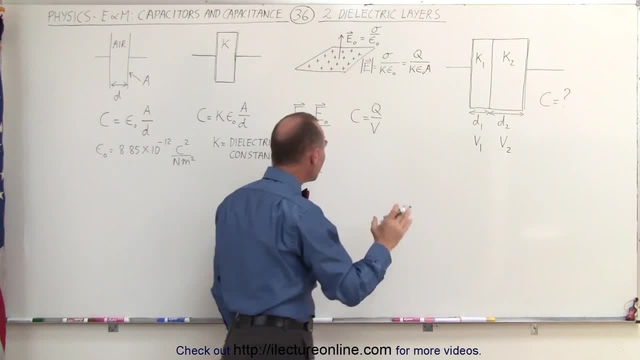 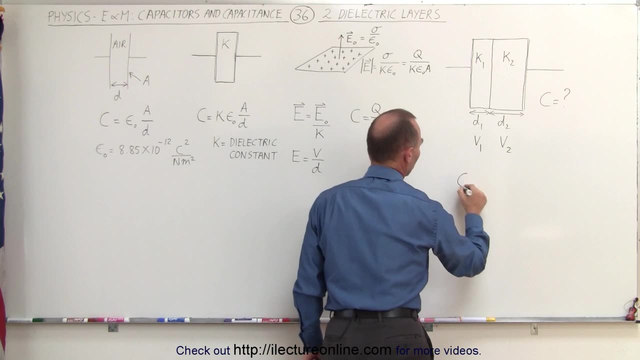 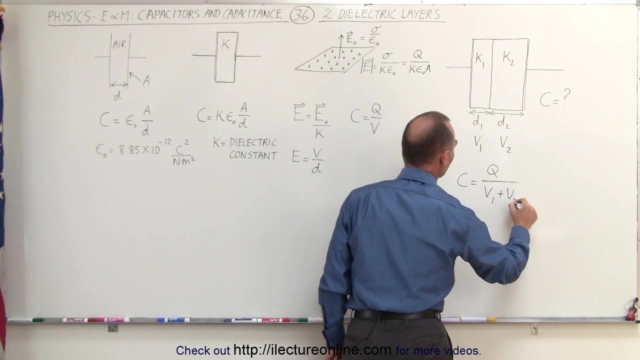 region here will have the potential difference of v2, which means that i should be able to find the capacitance by doing the following: the capacitance should be able should be able to be found by taking the total charge on the capacitor divided by the sum of the two voltages, because we can see that the total voltage will. 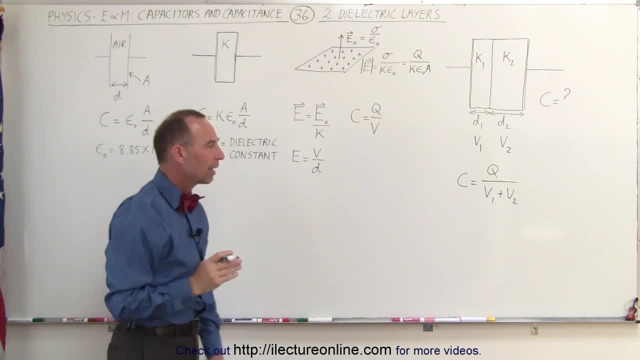 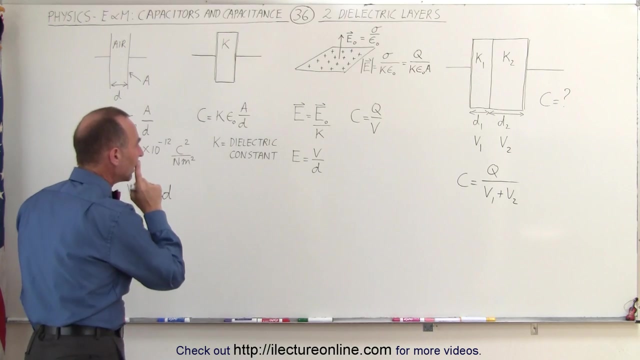 simply be the sum of the two. now can we figure out what v1 and v2 is equal to. going back over here, we can see that e is equal to v over d, or v is equal to the electric field strength. times d and electric field strength can be found by using. 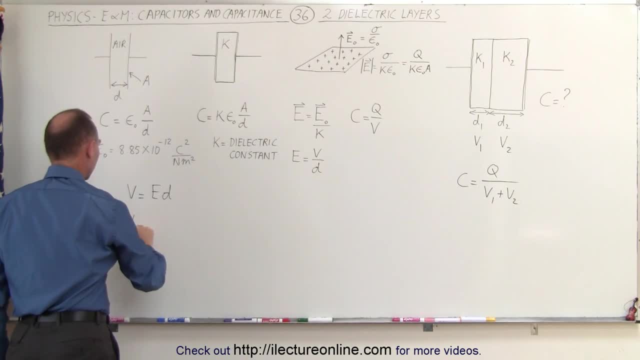 this equation right here, which means that the potential across the first layer is equal to the electric field strength about on the first layer times the distance of the first layer or the thickness of the first layer. and then we replace e sub 1 by that and we can say that this is equal to: 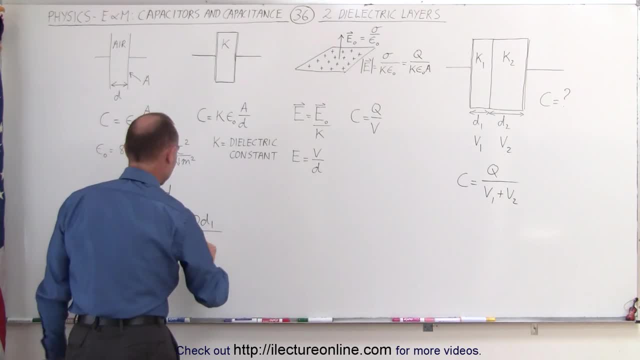 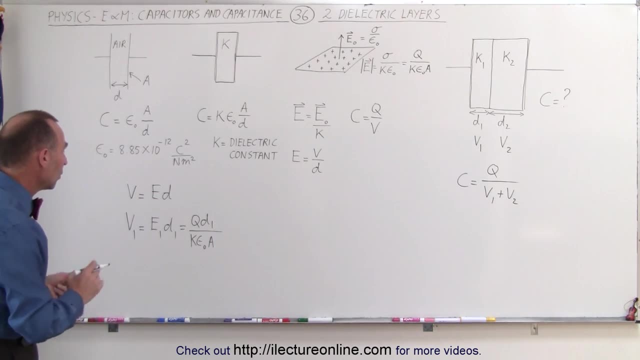 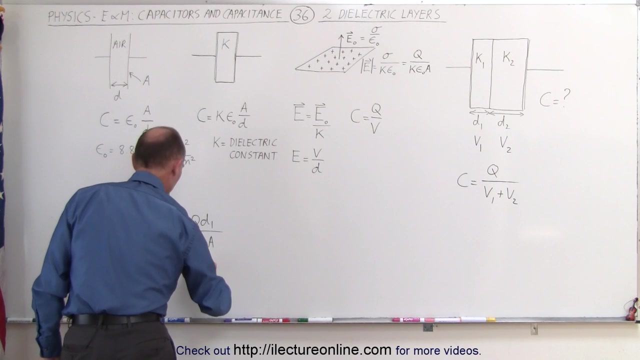 q times d1 divided by k epsilon sub naught times. a notice: that the area of the plates is the same for dielectrics. we can do the same for v2. v2 is equal to e2 times d2, which is equal to the charge q times d2. and i should call this k1 because 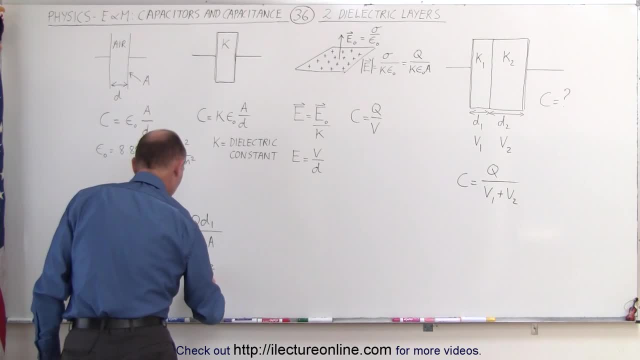 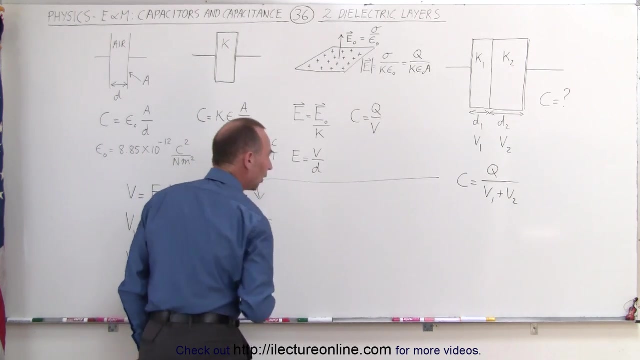 of course the dielectrics are different for both, and this would be q over times d2 over k2 times epsilon sub naught times a. i can then substitute those two values into my equation right here. so let me come over here, and i can then say that the capacitance of a capacitor with two 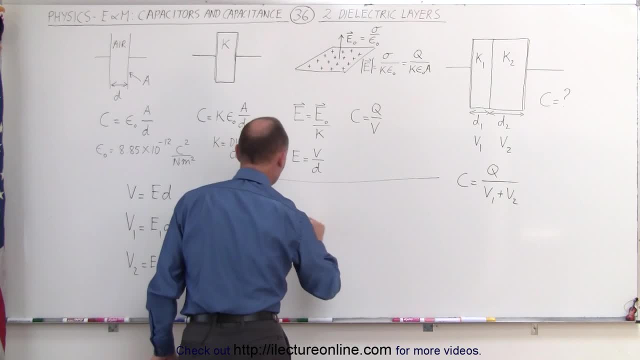 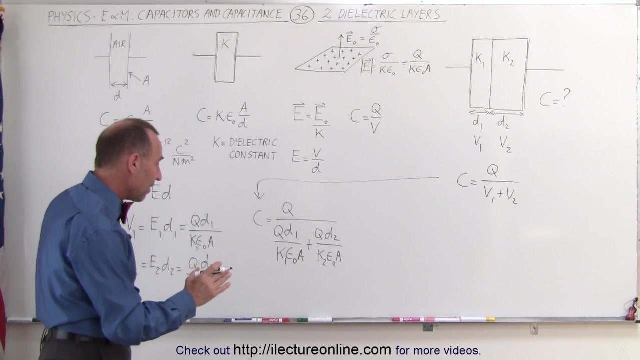 dielectric layers can be calculated to be Q divided by the sum of the two voltages, which is Q D1 over K1 epsilon sub naught times A. that would be for the first layer. that's the voltage of the first layer plus Q times D2 over K2 epsilon sub naught times A. Notice in the denominator: we can: 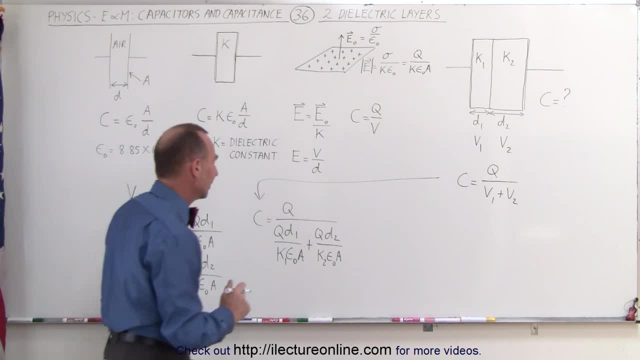 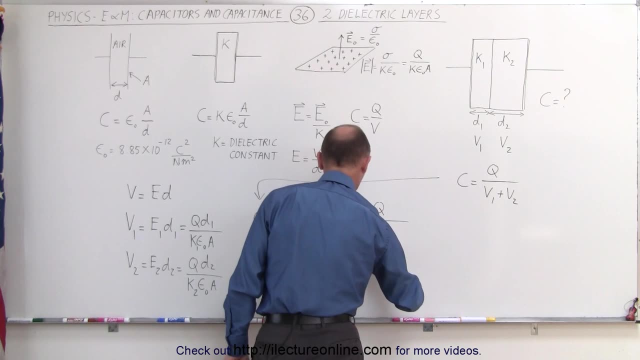 factor out a Q and epsilon sub naught N and A. Let's do that. so this is equal to Q divided by Q divided by epsilon, epsilon sub naught times A. so I can factor it out and I have left D1 over K1 plus D2 over K2.. Notice that this Q and this Q cancels out this becomes one. I can bring this. 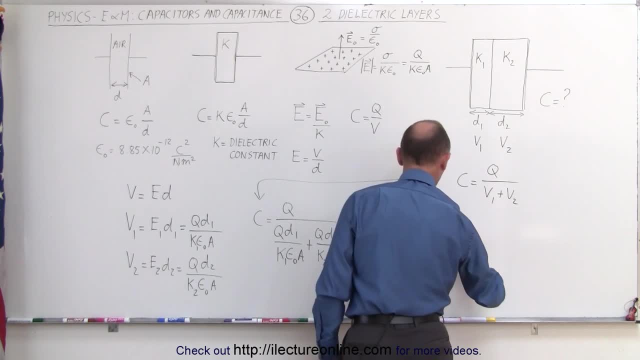 to the numerator, and so finally, we can say that the capacitance with two layers is going to be equal to D1 over K2.. epsilon sub naught times A, divided by D1 over K1, plus D2 over K2, and that's how you find the. 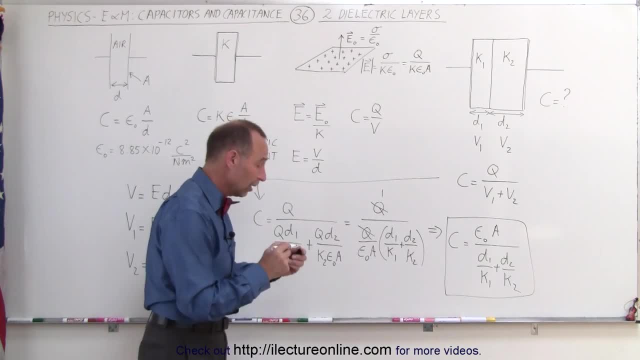 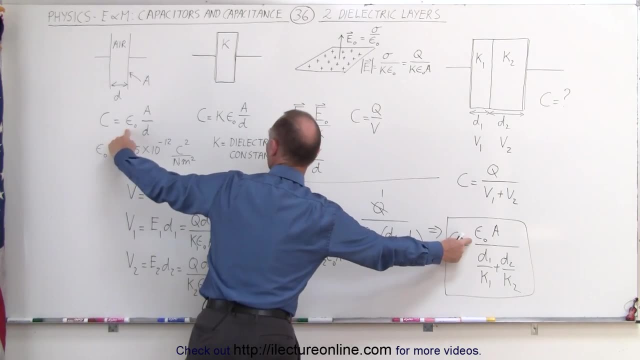 capacitance of the capacitor that has two dielectric layers in it. Now let's compare that equation to our original equation. Notice the capacitance is equal to E epsilon sub naught times A divided by the distance. Now notice that the distance will be weighted depending upon the 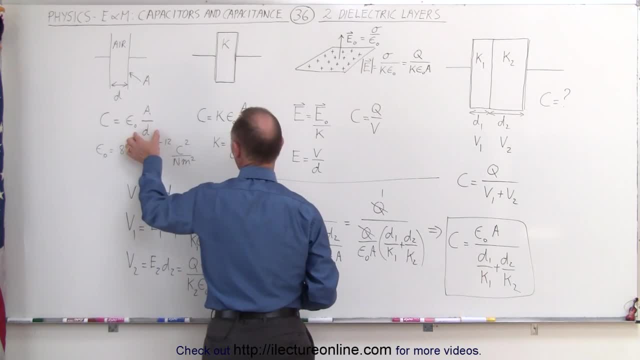 dielectric layer. So this is equal to E epsilon sub naught times A divided by the distance. The distance will be the dielectric constant, and so we sum up the distances. so D total will simply be D1 plus D2, but depending upon the dielectric constant they will have a different weight factor.